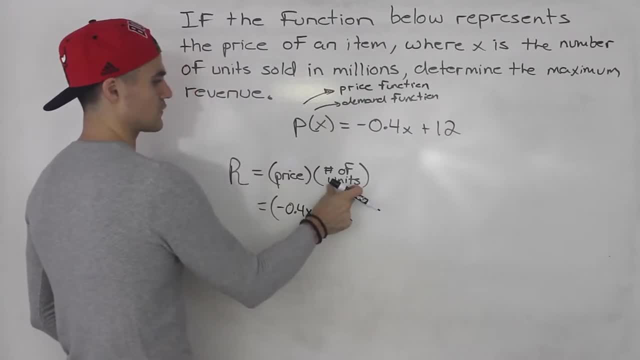 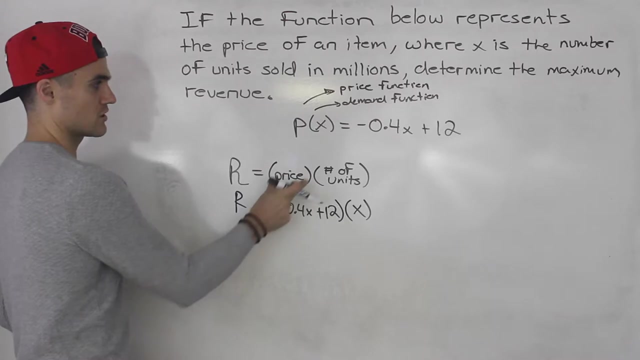 plus 12.. But we need something for the number of units. And notice how x is the number of units sold. It's in millions, but the number of units is just represented by x. So this here is the revenue function, The price function, multiplied by x, the number of units sold. 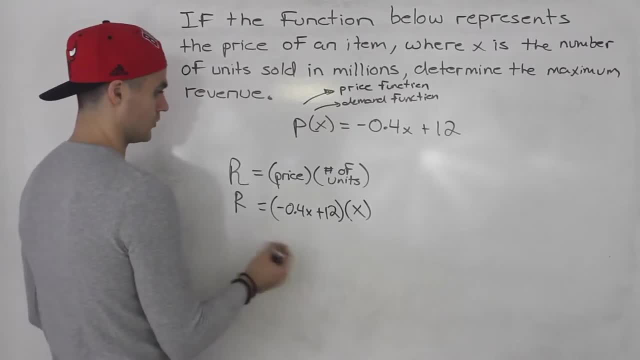 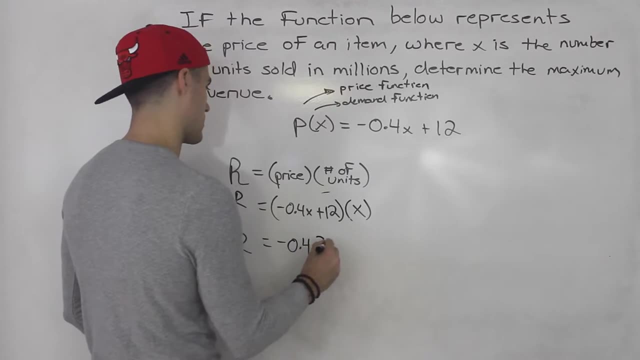 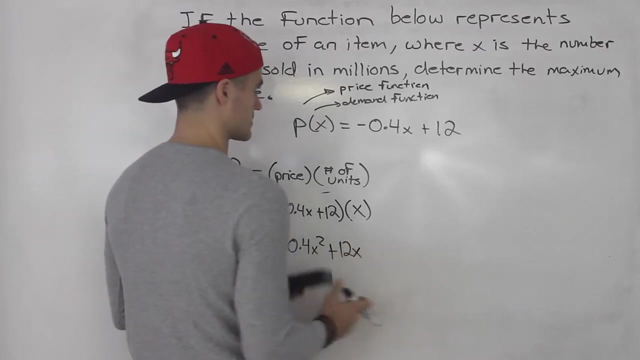 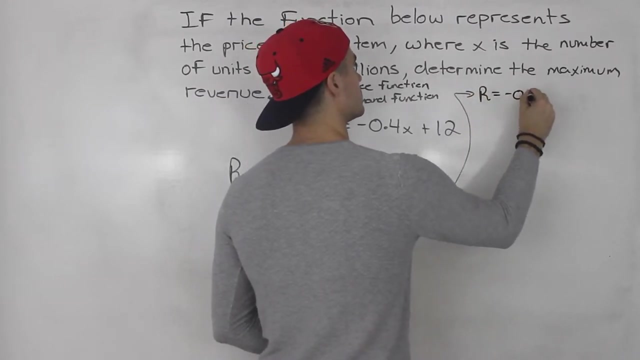 And now they're asking for the maximum revenue. What we can do multiple ways to do this, I'm going to distribute the x inside the bracket, So I'll have negative 0.4x squared plus 12x. So let's rewrite that up here actually. So we got r equals negative 0.4x squared plus 12x. 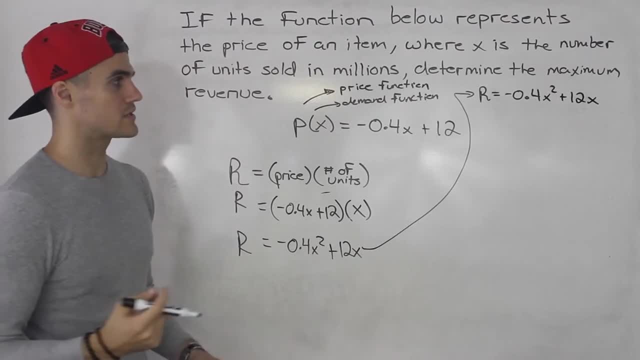 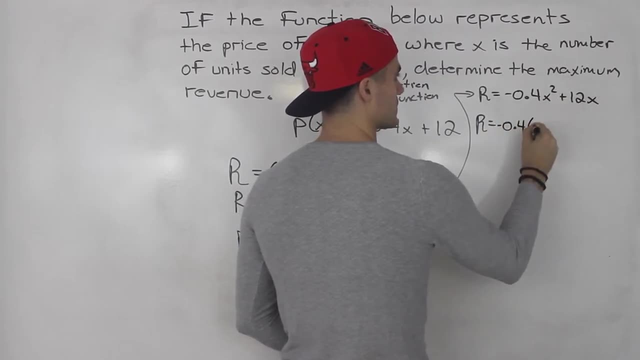 And now, with this revenue function, we have to find the maximum revenue. So let's complete the square So we can factor out a negative 0.4 from both of these. So we'd have x squared minus 12. divided by negative 0.4 gives us negative 30x. 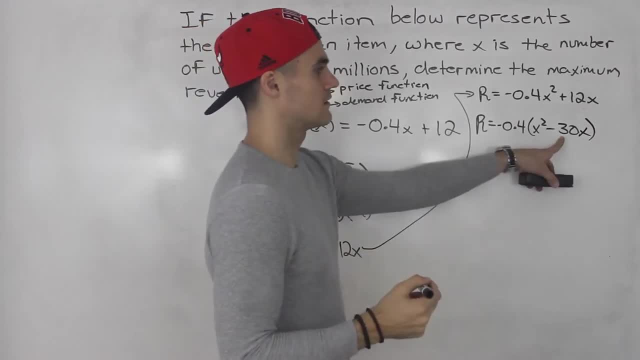 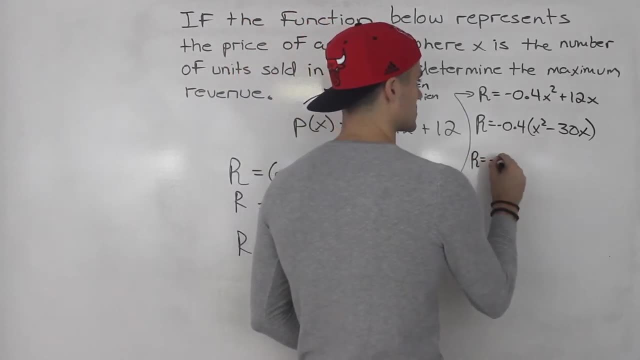 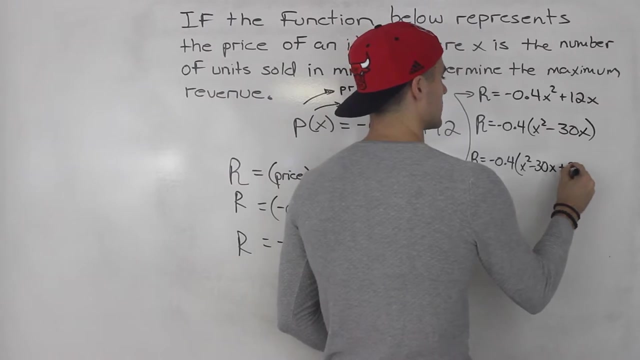 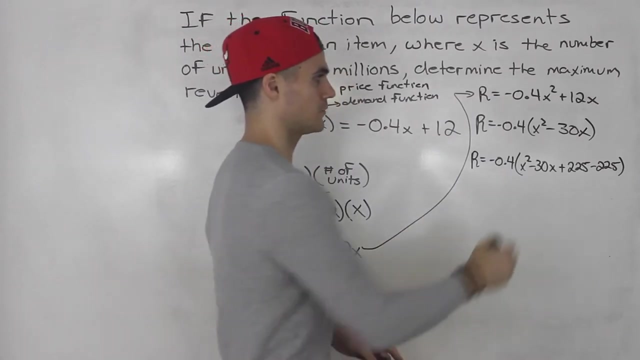 Like that. So then we would take negative 30 divided by 2, negative 15, square it, that gives us 225.. So we'd have r equals negative 0.4 x squared minus 30 x plus 225, minus 225, like that. And then, continuing on, we take out the negative 225 from the bracket and multiply it. 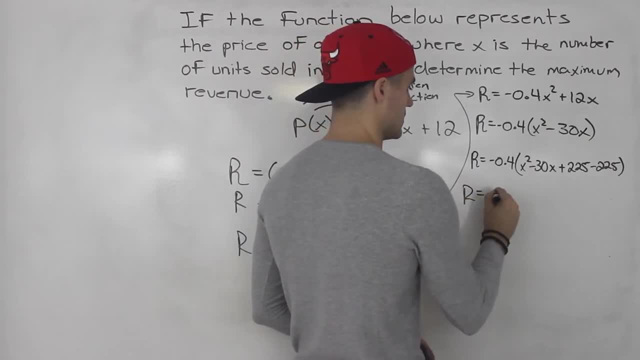 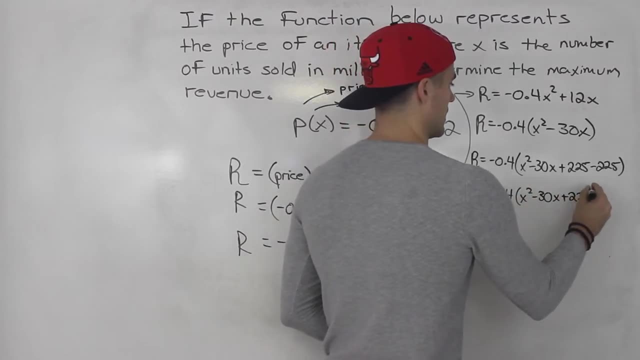 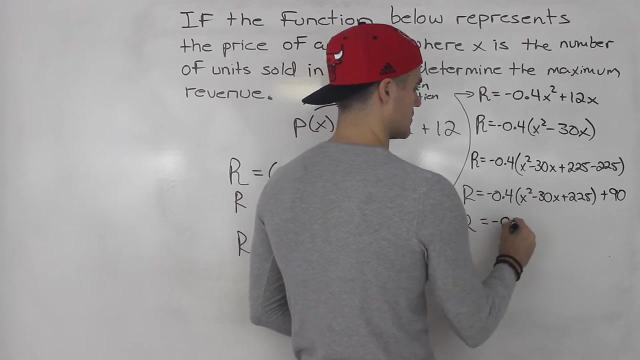 by negative 0.4 outside. So we'd have negative 0.4 x squared minus 30 x plus 225.. Negative 225 times negative 0.4 gives us positive 90.. And then this here, this bracket is going to factor into x. 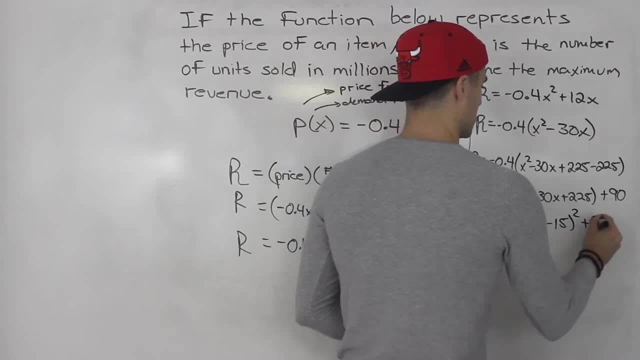 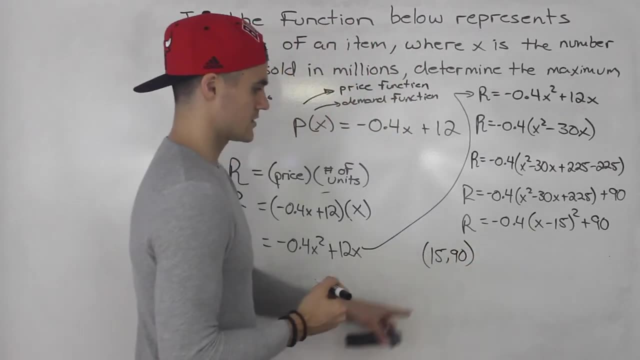 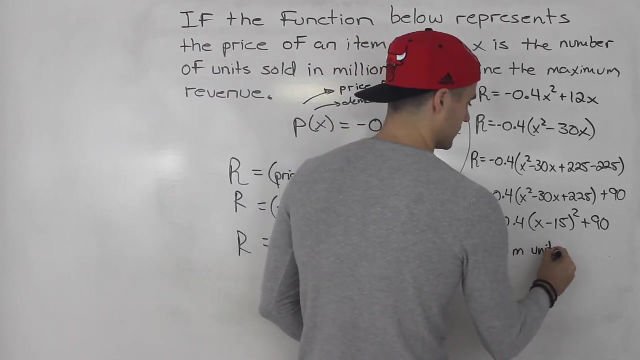 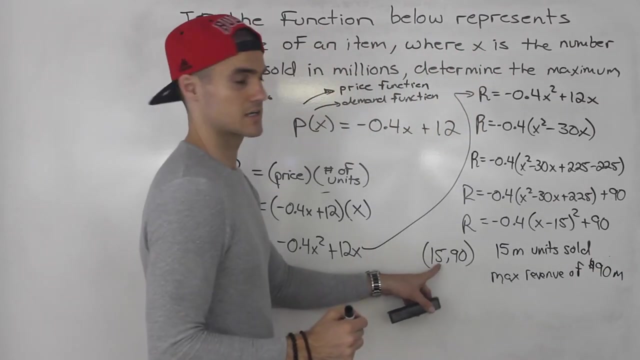 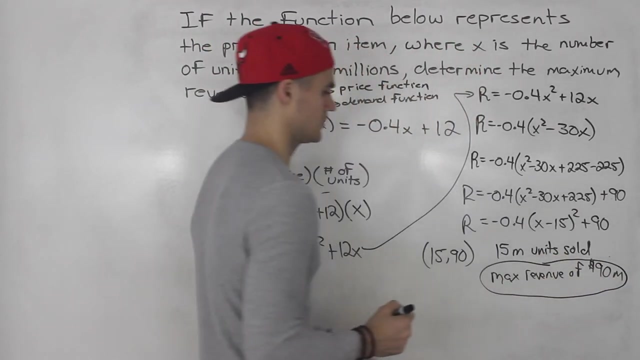 minus 15, squared plus 90.. Vertex here is 15 and 90. So this 15 million units sold gives us a max revenue of 90 million. That's what this vertex means with this function here. So really, what they were asking for is this part, the maximum revenue of 90 million, just the y value.